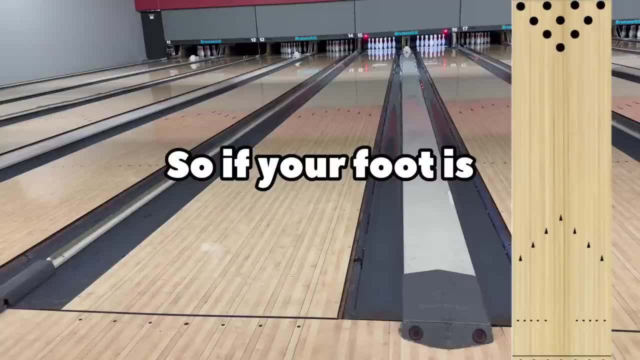 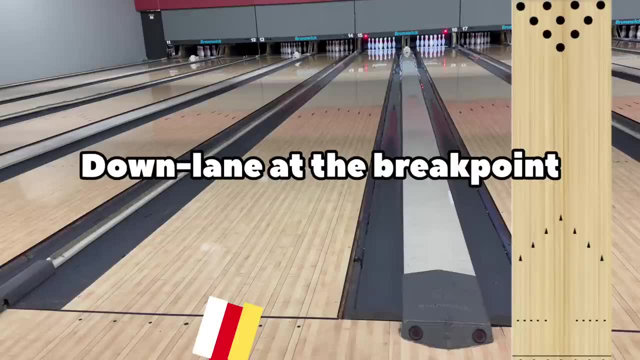 have no idea what happens after the arrows. So if your foot is one or two boards off where you slide, you can hit your target at the arrows, but it can be three or four boards off down lane at the break point and give you a drastically different result. 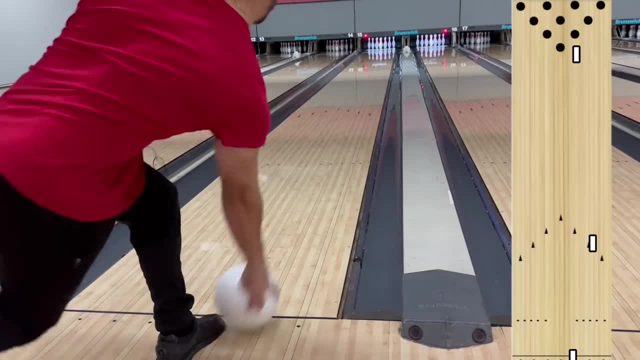 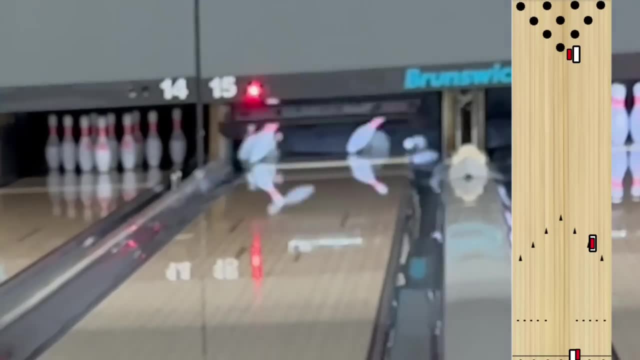 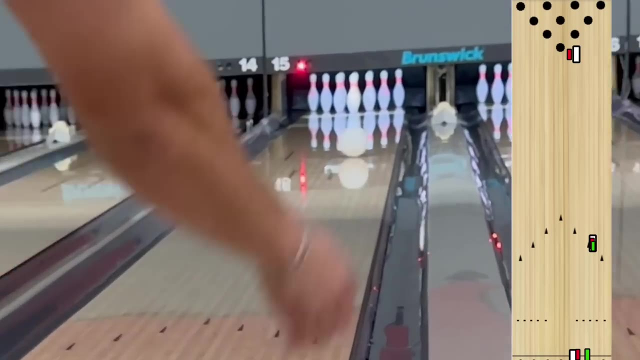 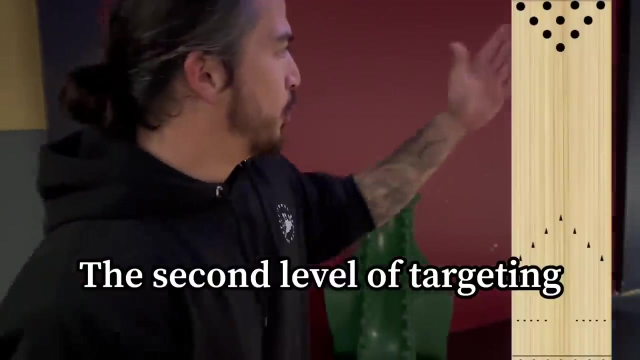 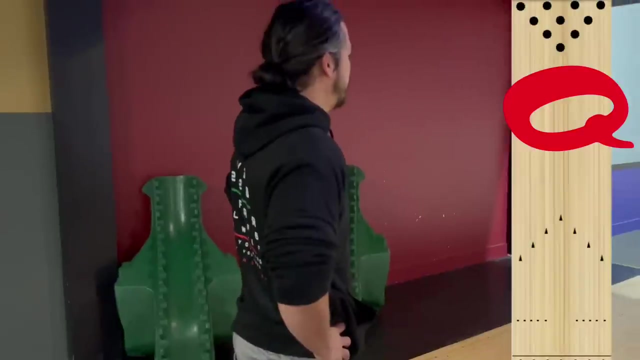 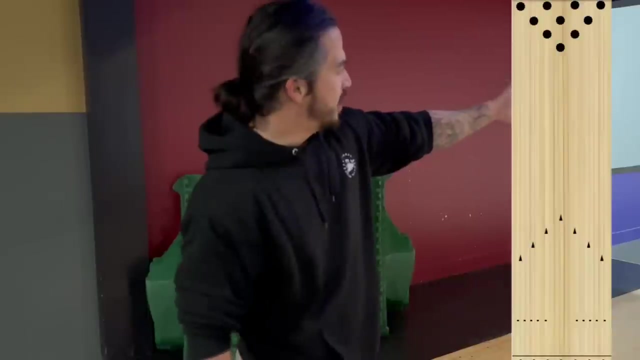 So the second level of targeting is targeting your break point, which is about 40 feet down the lane where the oil pattern ends, Generally on a house shot. you want to get to around eight to 10 at the end of the pattern, which is right by that little brown marker about 40 feet down the lane. 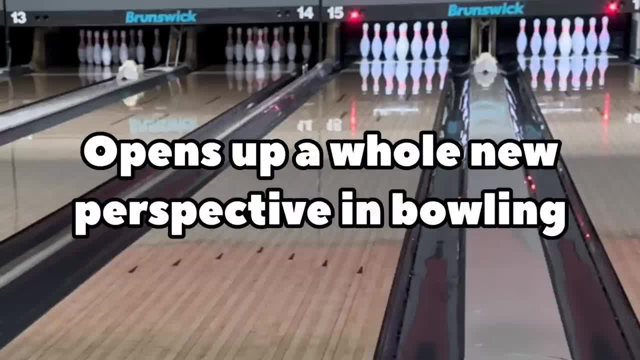 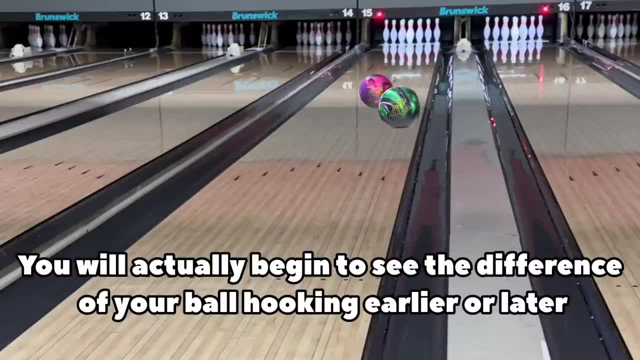 Targeting the break point opens up a whole new perspective in bowling. When you target the arrows, you don't really see what happens after that. But once you start to see the break point you will actually begin to see the difference of your ball hooking earlier. 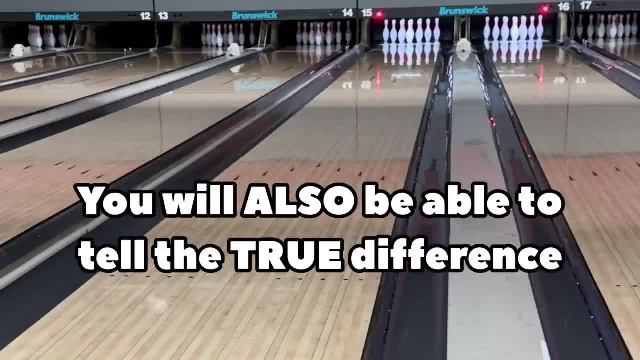 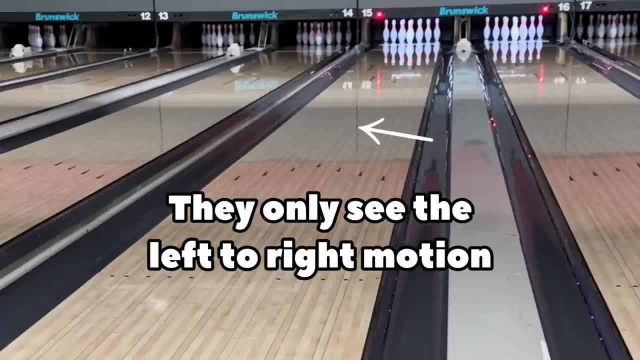 or later You will also be able to tell the true difference between a strong ball and a weak ball. When most bowlers watch a bowling ball go down the lane, they only see the left to right motion and they can't see the front to back motion. A strong ball will actually begin to hook earlier. 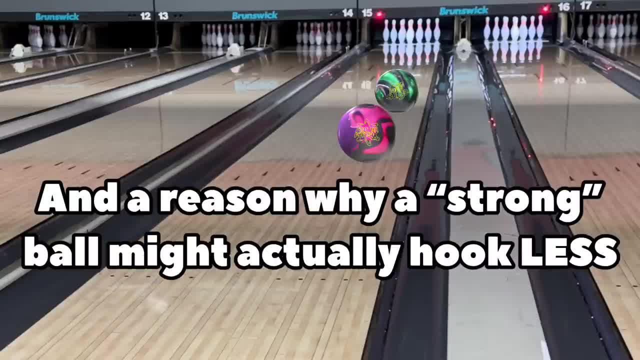 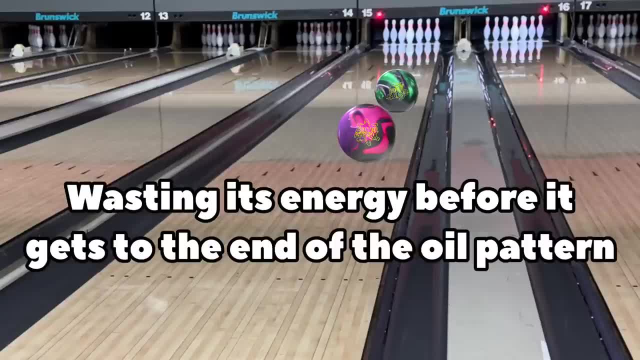 on the lane than a weak ball. And the reason why a strong ball might actually hook less than a weak ball left to right is because it's hooking too early, wasting its energy before it hits the end of the oil pattern, while the weak ball retains it and comes off the pattern. 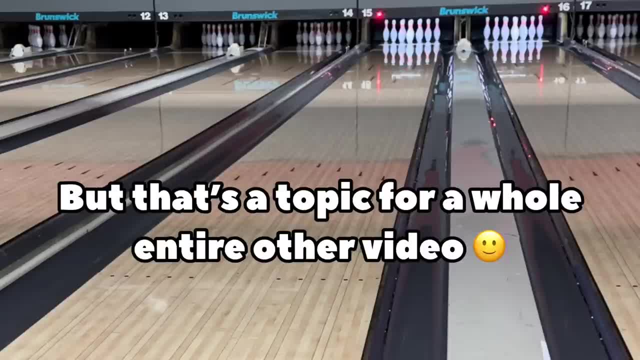 a lot sharper, But that's a topic for a whole entire other video. Now the third level of targeting is targeting your ball. So if you're a strong ball, you want to target your ball as far as possible, And what I currently do now is I'll target my break point. 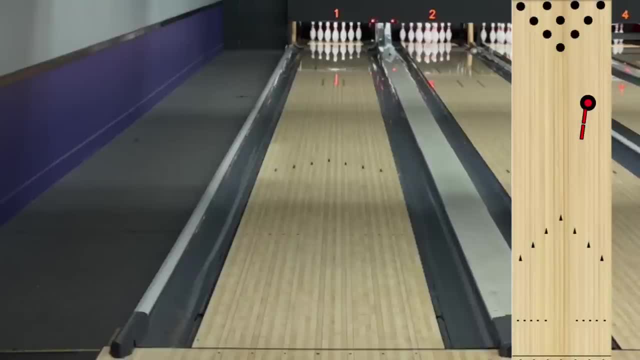 and I'll draw a line back to the arrows. So for this shot, I'm getting it right to the right of that marker. I'm going to draw a line back to just left of third arrow. So about 17 at the arrows and